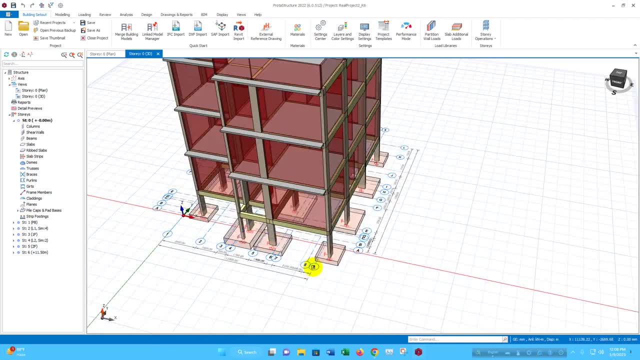 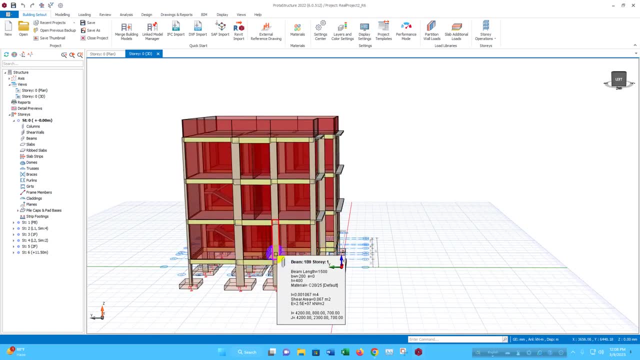 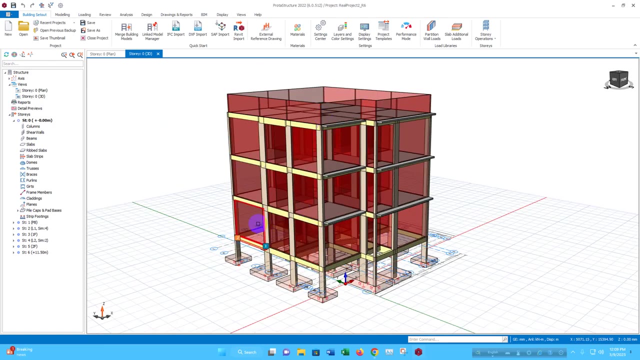 In this update this new feature has been added. Along with the structural design, we have to do the formwork design also. This formwork design has been made very easy by Protai. So now go for the formwork design. First I can go for column formwork design. 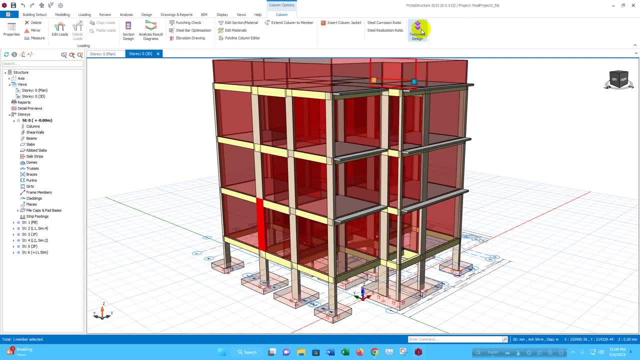 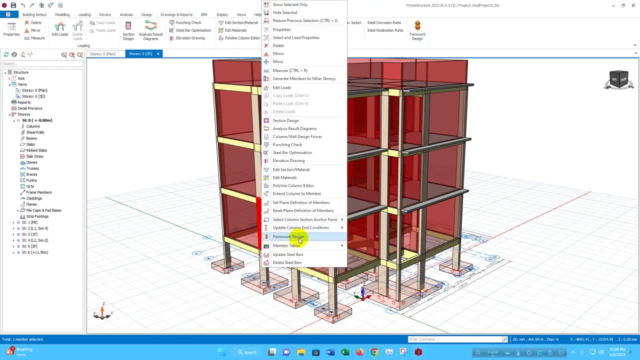 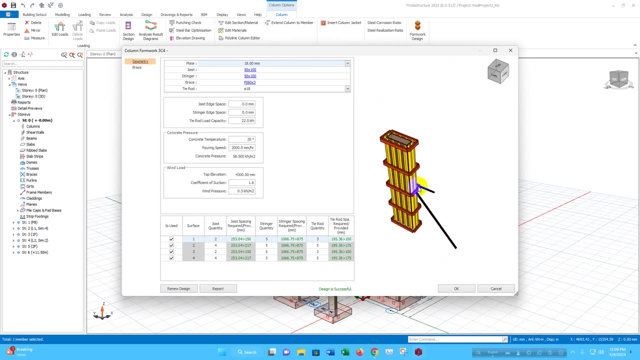 Here I have selected the column. Here also we are getting the option for formwork design. Or if we go for right click here we will get formwork design. Click on this Here according to the size of the column. the formwork has been generated automatically Here: joist size. 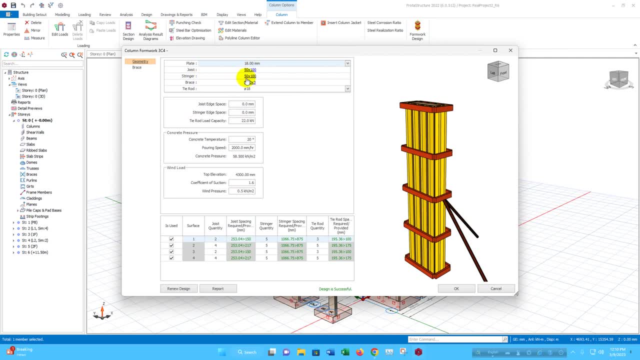 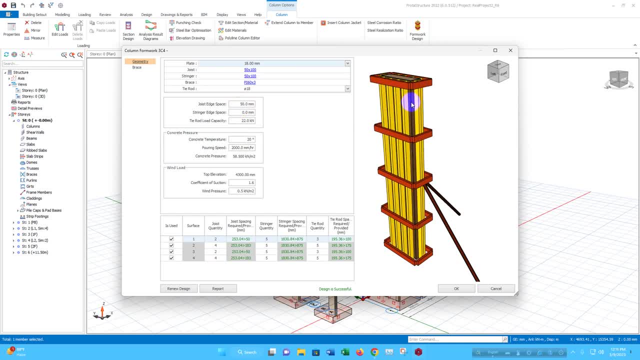 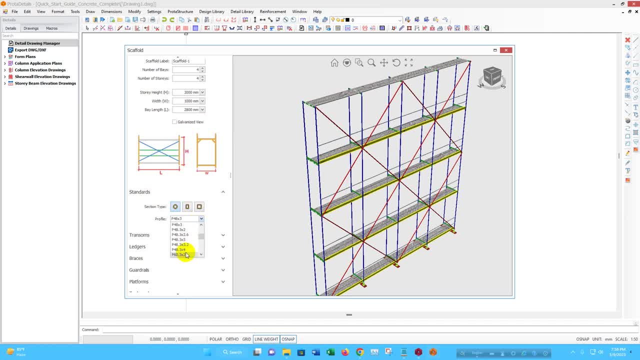